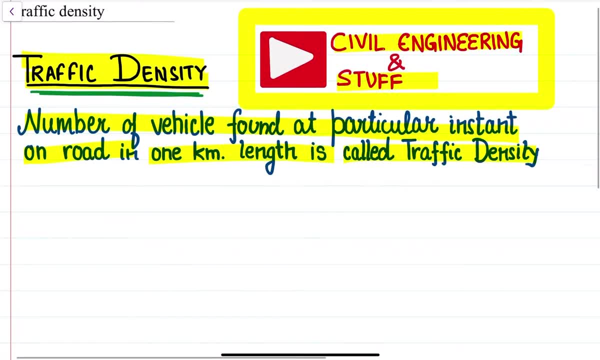 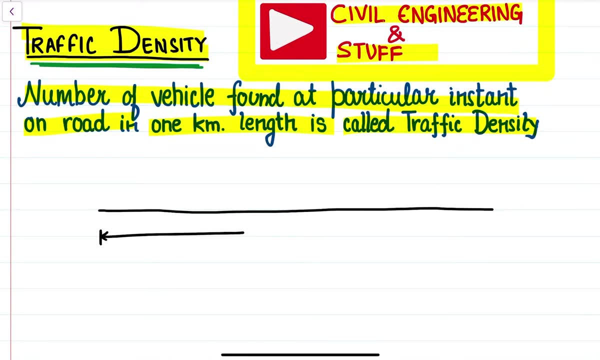 instant on the road in 1 kilometer length. What does this mean? This means that in a steady stretch of traffic density, the number of vehicles found at a particular instant on road in 1 kilometer length in a steady stretch of 1 kilometer. In a steady stretch. 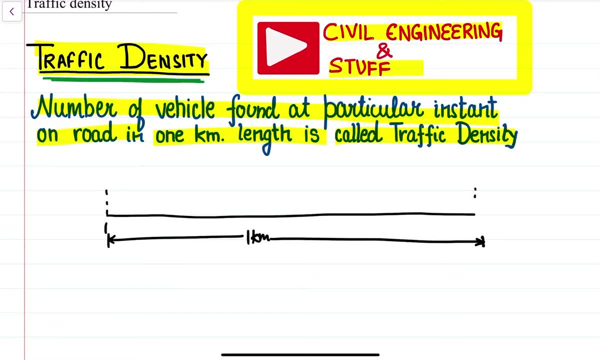 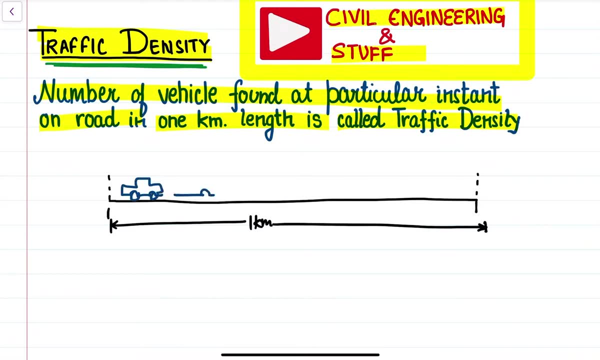 of 1 kilometer. how many vehicles are occupying this section of the road? So, how many vehicles are occupying this 1 kilometer section of the road is what we call as the traffic den. imagen- traffic density. This is what we call as the traffic density, So this means the unit of 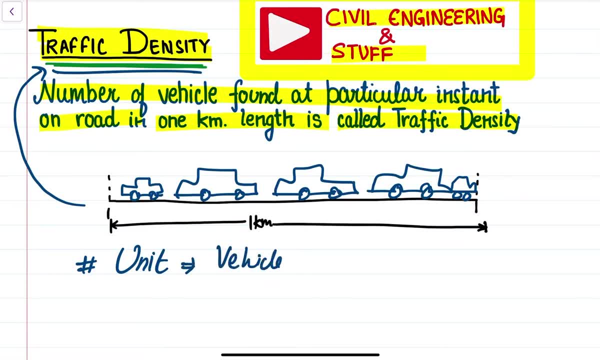 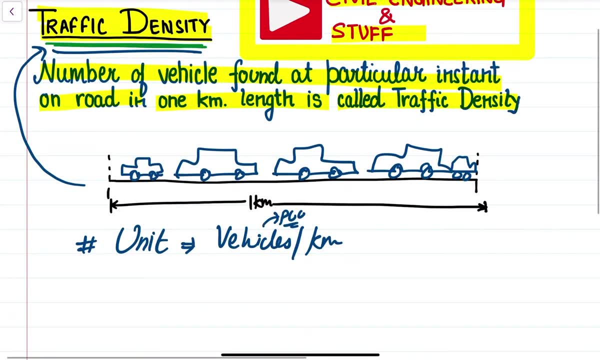 traffic density will be vehicles per kilometer, vehicles in ECU, So how many vehicles are occupying one kilometer length of the road is called as the traffic density. So one thing that you should notice or compare between the traffic volume, traffic capacity and this: 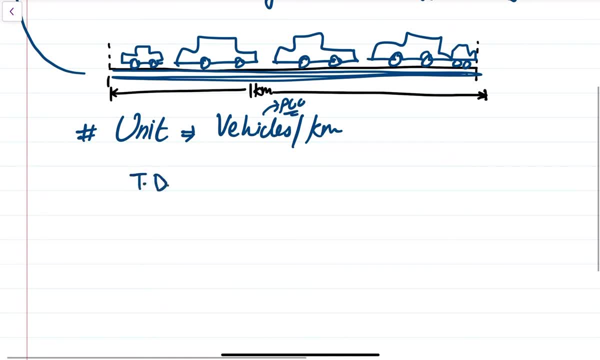 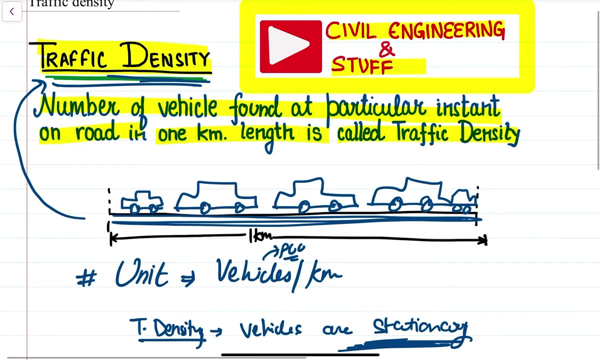 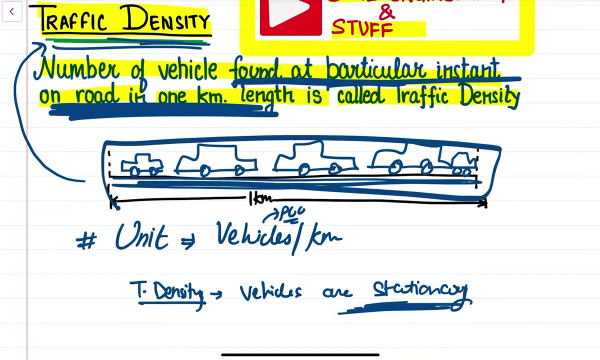 traffic density is that in traffic density the vehicles are stationary. If you look into the definition again, the vehicles are occupying one kilometer. One kilometer section of the road the vehicles are found at a particular instant. so we are looking at the stationary occupancy, we are not looking at the number of vehicle. that 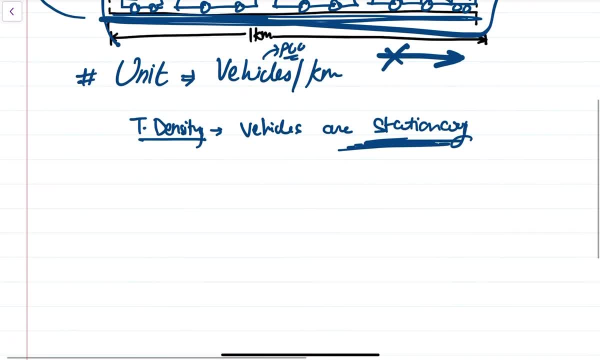 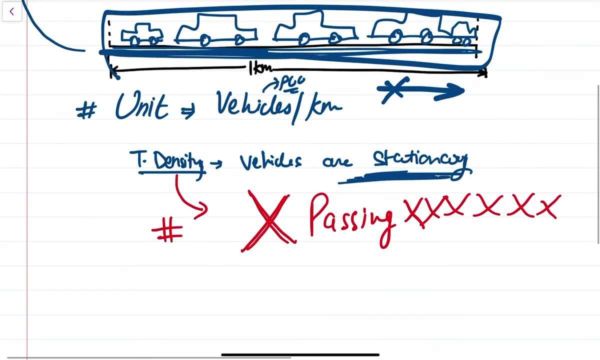 are passing one kilometer section of the road. I will just write it down. It's a very important and a very confusing thing that in traffic density we are not looking into the vehicles that are passing the one kilometer section of the road. This is not the case. We are. 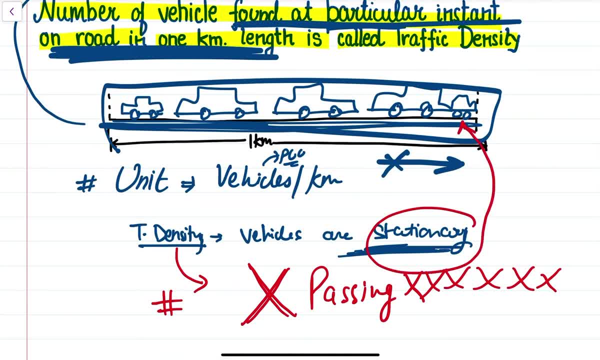 looking at the vehicles that are occupying this one kilometer section of the road at any particular instant of the time. it can be the peak hours, it can be the mid peak hours, or it can be the low traffic volume time like 2 am- 3 am. 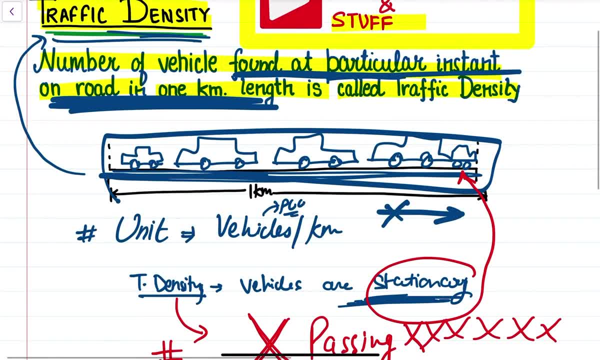 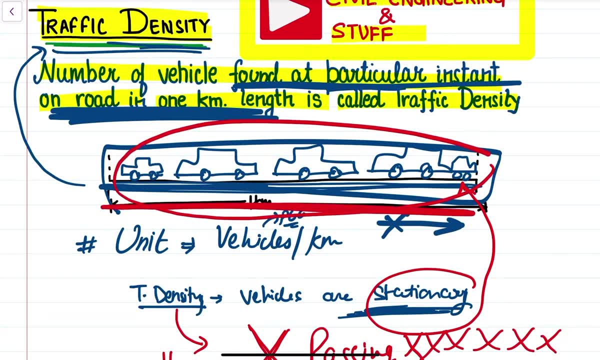 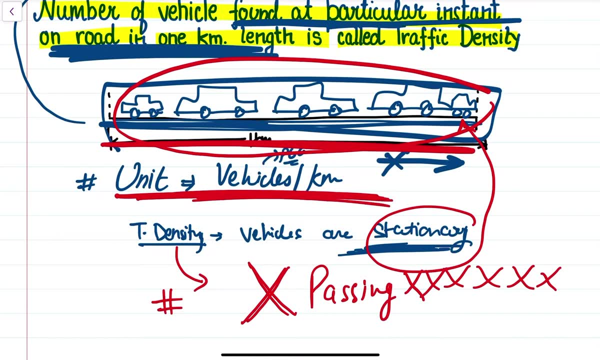 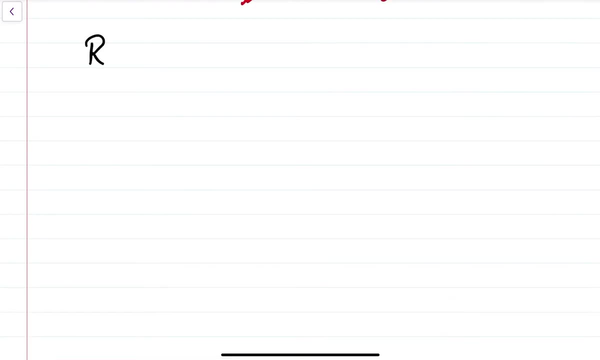 in the morning. okay, so the traffic density is the number of vehicles occupying a section of the road, one kilometer section of the road at any point of time. so the unit of traffic density is vehicle per kilometer. okay, unit is vehicles per kilometer. so what is the, what is the relationship, what is? 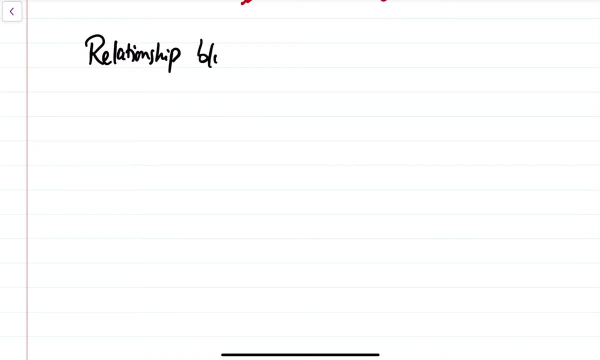 the relationship between? what is the relationship between traffic volume, traffic speed and traffic density? now you see, we are talking about it: traffic as a whole. so this is a macroscopic, this is a macroscopic parameter, when we we have already discussed in the video what is macroscopic and microscopic parameter. 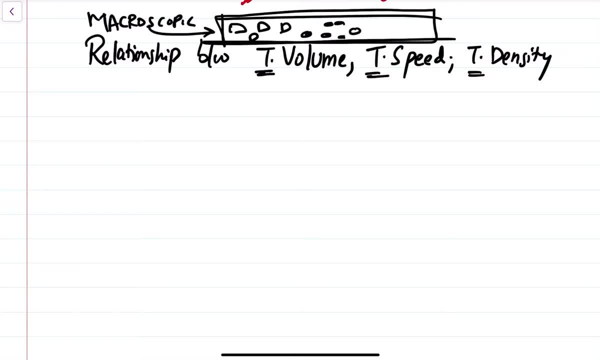 so when we are looking at a traffic as a whole, it is called as the macroscopic parameter, right? so the relationship between traffic volume, traffic speed and traffic density is that your traffic volume, your traffic volume, is equal to traffic speed. multiplied by traffic density, traffic volume is equal to. 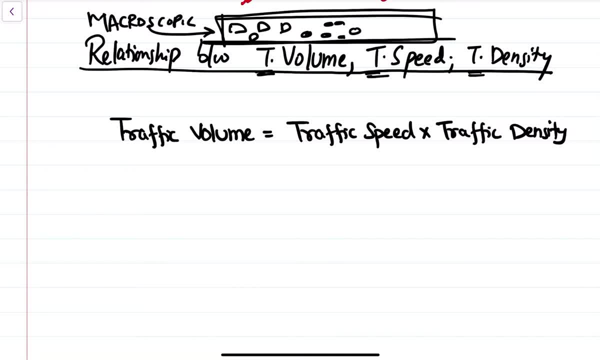 traffic speed multiplied by traffic density. so we know the unit of traffic volume is equal to the distance of the road. vehicle per unit time time can be hour. vehicle per unit time time can be hour. vehicle per unit time time can be hour. series distance: it can be kilometer or. 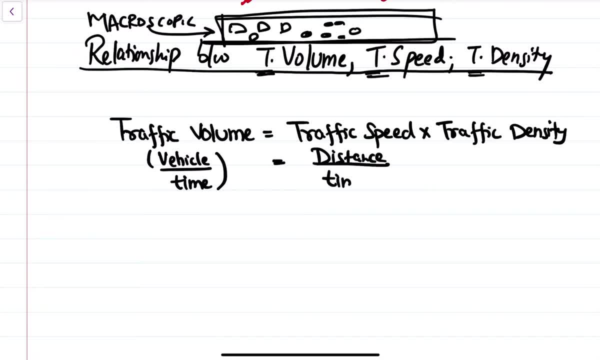 series distance. it can be kilometer or series distance. it can be kilometer or meter distance per unit time density. we meter distance per unit time density. we meter distance per unit time density. we have discussed is a vehicle per have discussed is a vehicle per have discussed is a vehicle per kilometer. that is the distance right. 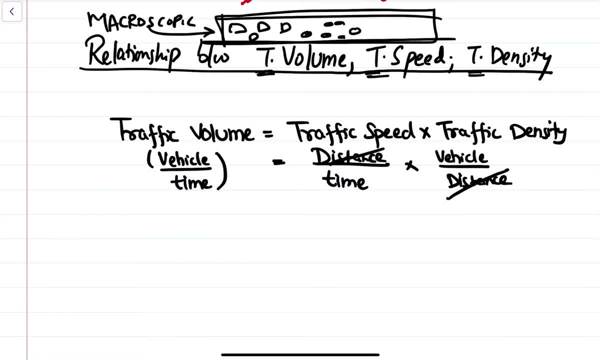 kilometer, that is the distance, right. kilometer, that is the distance right. affection of the road, the distance. so you, affection of the road, the distance, so you affection of the road, the distance. so you can see we this is, can see we this is being cancelled. So, vehicle per unit time: vehicle per unit time. the units are matching.